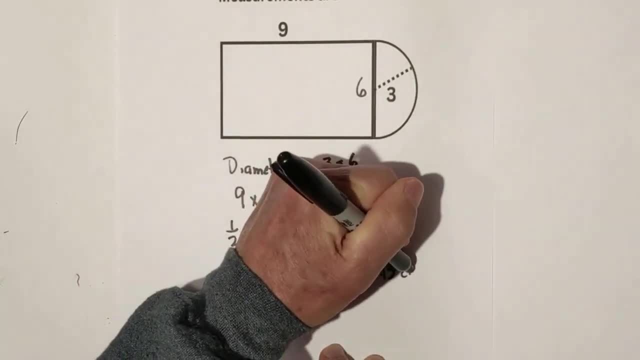 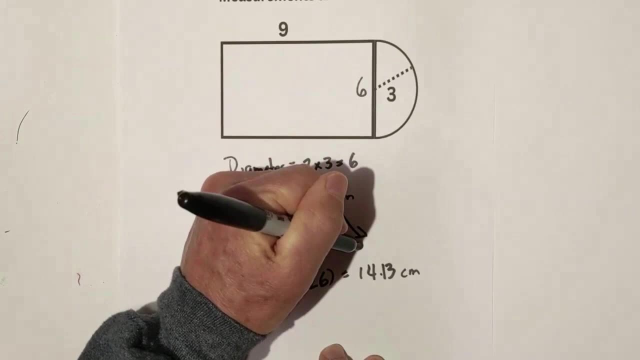 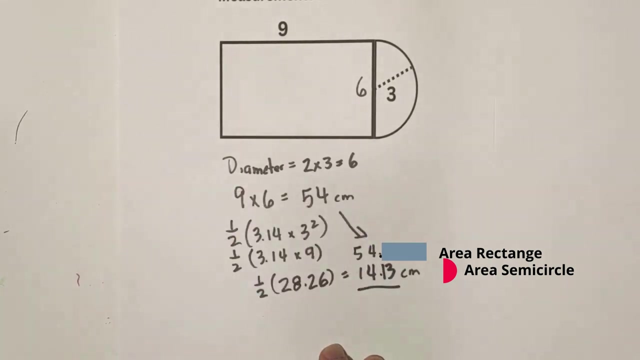 oops, sorry about that. okay, remember, this is in centimeters also. now all we do is we add this 54 that we got from here, plus the. this is the rectangle, this is the semicircle. when you add these together, you just multiply. they're gonnaheardisa the youlls because you just subtractじゃあ, if you, Derek. 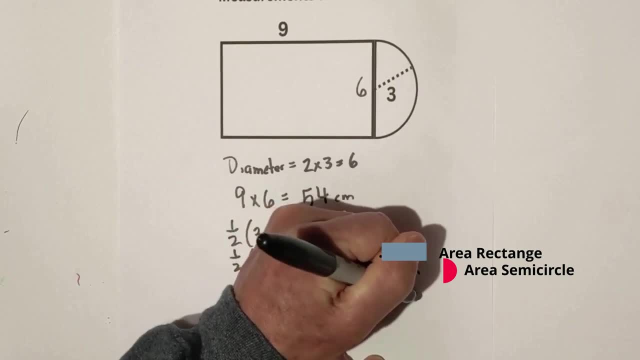 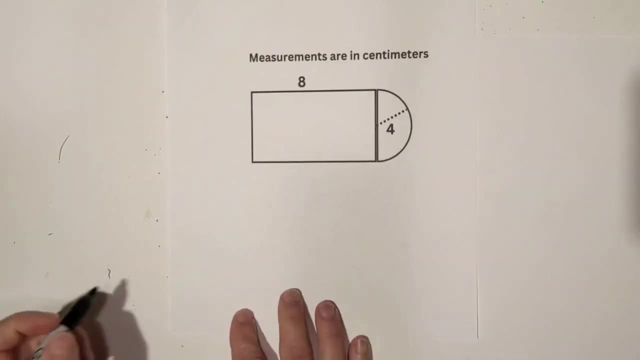 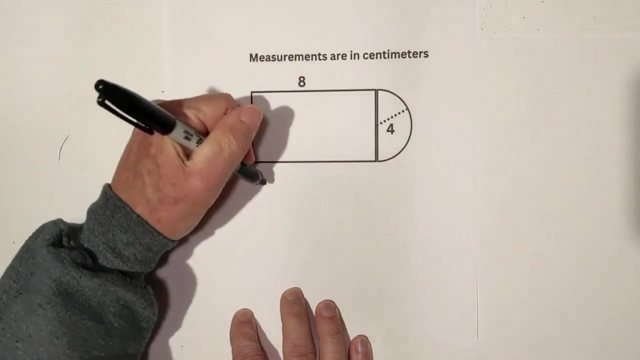 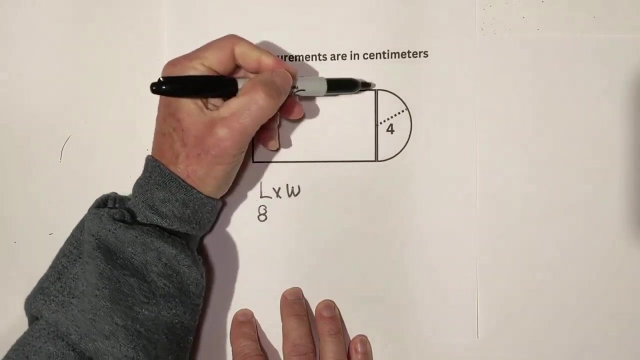 get 68.13, and area is always squared. okay, let's look at this second one again. we have a rectangle and a semicircle, and so what we need to do is the area of a rectangle again is length times width. so we're going to go 8, but we don't have the width given. however, we do have the radius and we know. 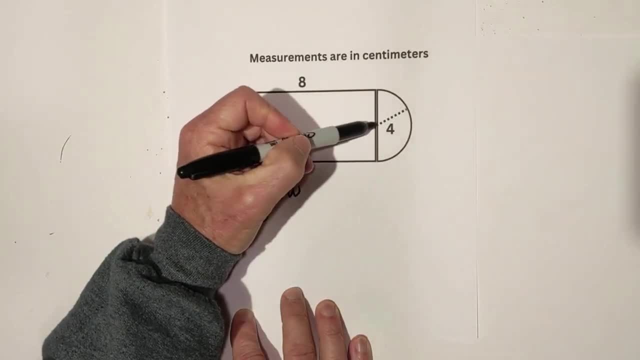 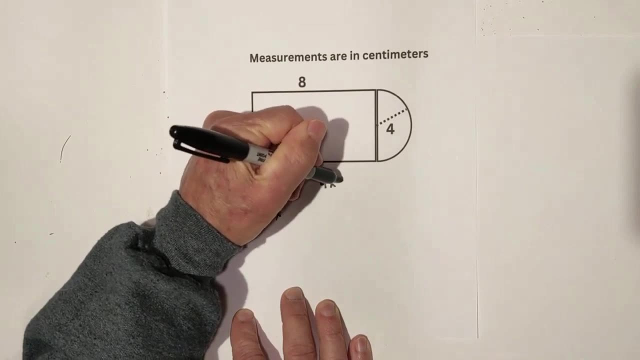 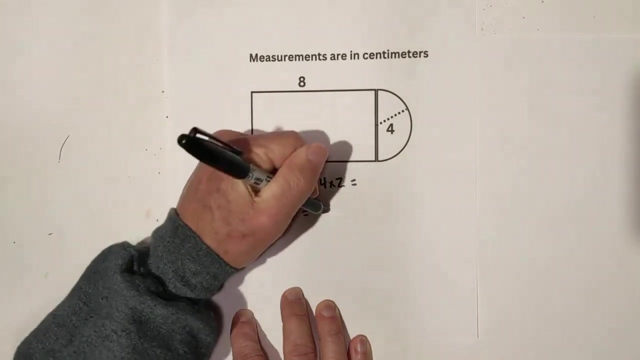 that the radius is going to be half of this line right here, because it's the diameter of the semicircle. so all we have to do is go 4 times 2, because the diameter is 2 times the radius, and that equals 8. when we multiply 8 times 8, that gives us 64, and the measurements are in centimeters. 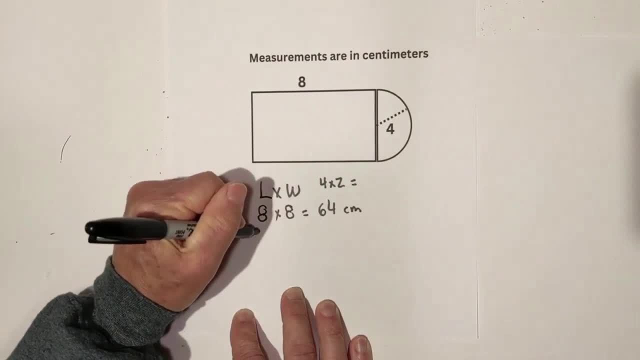 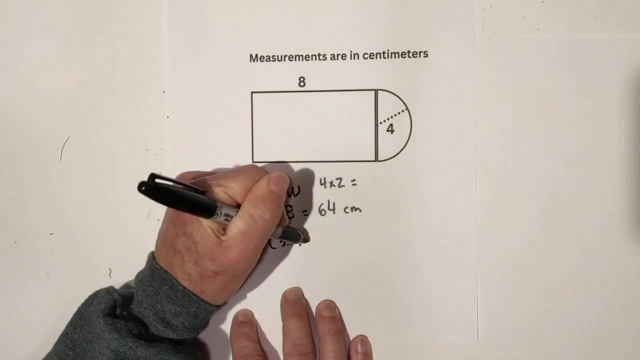 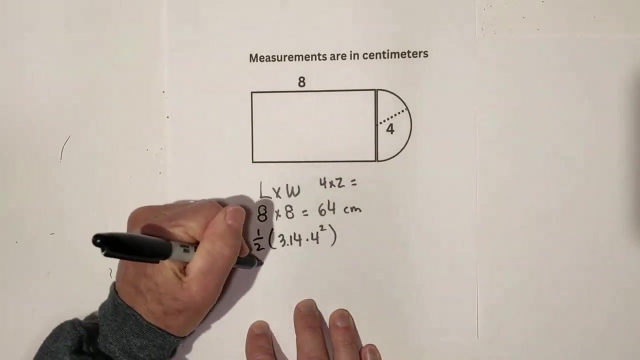 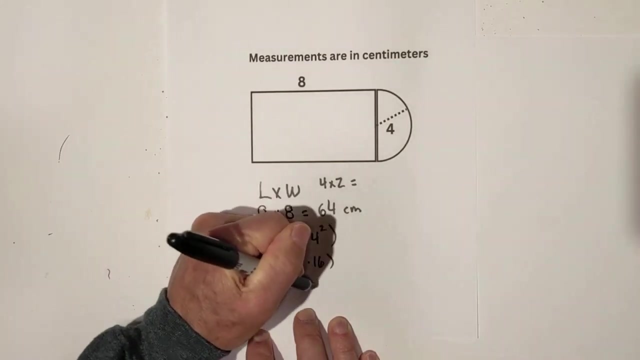 so now let's focus on this semicircle, and we can use one half times pi. i'm going to use 3.1, 4 times the radius squared, so we have 4 squared. let's work what's in the parentheses. first, one half times 3.14 times 16. okay, when you multiply 3.14 times 16, that gives me us 50.24. now i'm going. 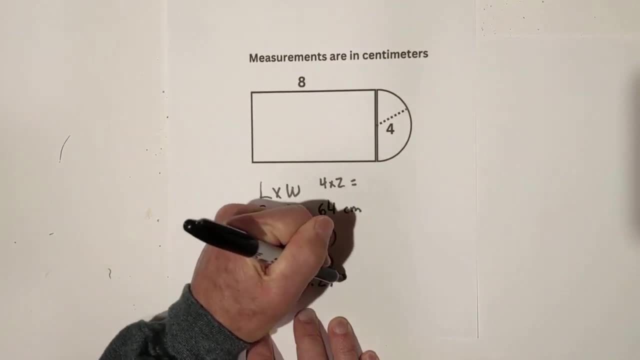 to multiply that by one half and that gives us 64, and the measurements are in centimeters, which you 25.12, so this will be in centimeters. so now all we need to do is add these two together. i'm going to bring down the area of the rectangle. that equals 64.00. okay, so far, so good. when we add: 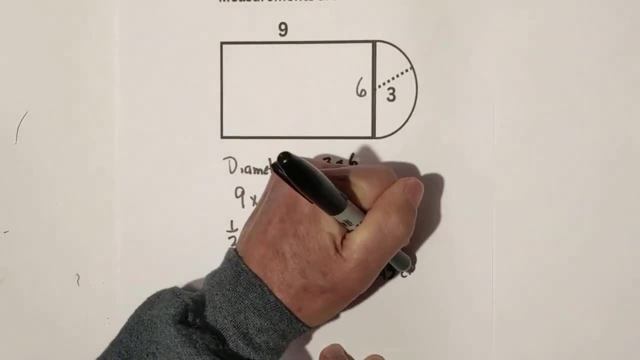 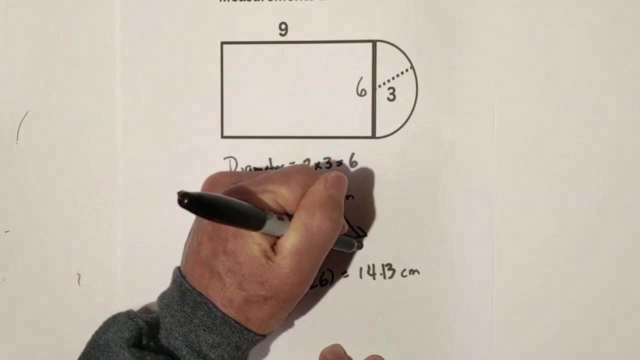 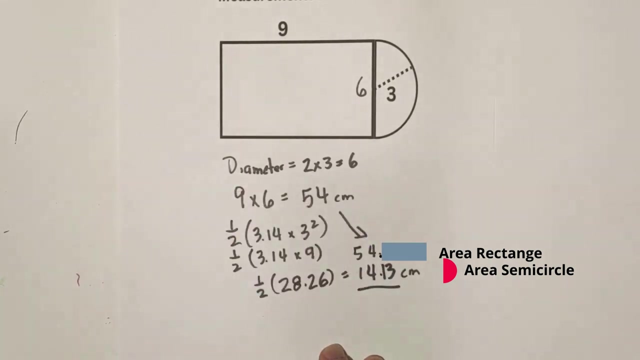 oops, sorry about that. okay, remember, this is in centimeters also. now all we do is we add this 54 that we got from here, plus the. this is the rectangle. this is the semicircle. when you add these together, you change what we get in the semicircle. so we get this one half plus. this is the rectangle. this is the semicircle. when you add these together, you. 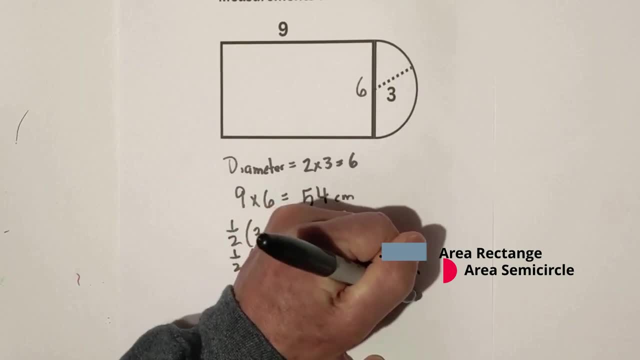 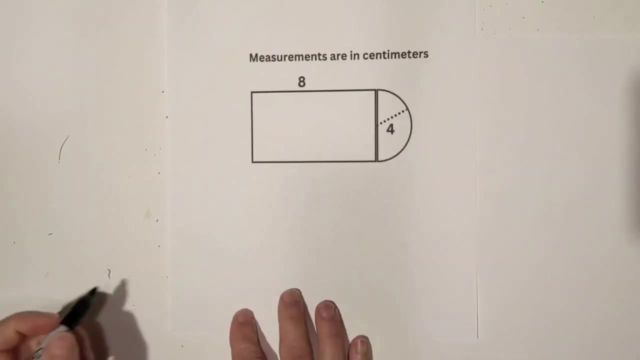 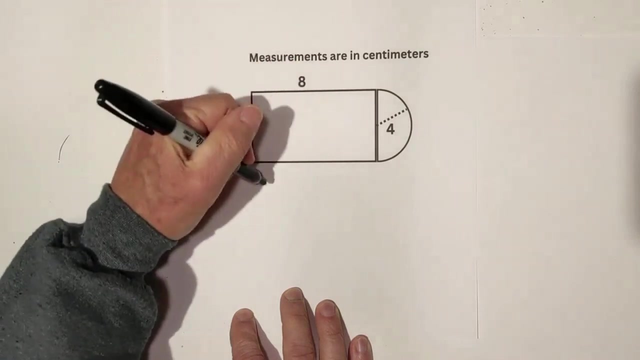 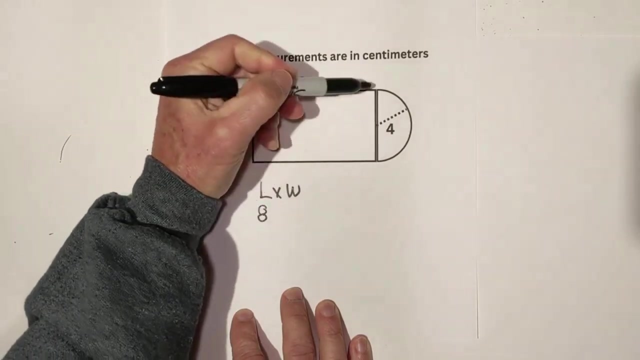 get 68.13, and area is always squared. okay, let's look at this second one again. we have a rectangle and a semicircle, and so what we need to do is the area of a rectangle again is length times width. so we're going to go 8, but we don't have the width given. however, we do have the radius and we know. 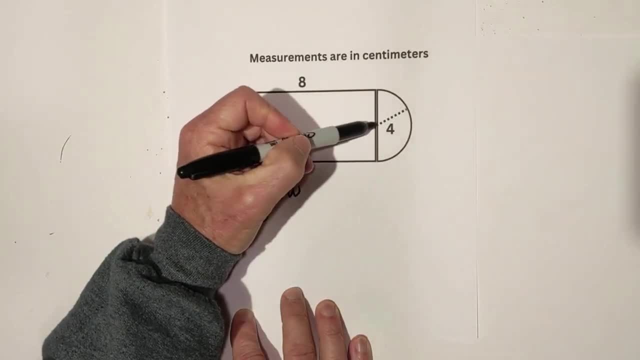 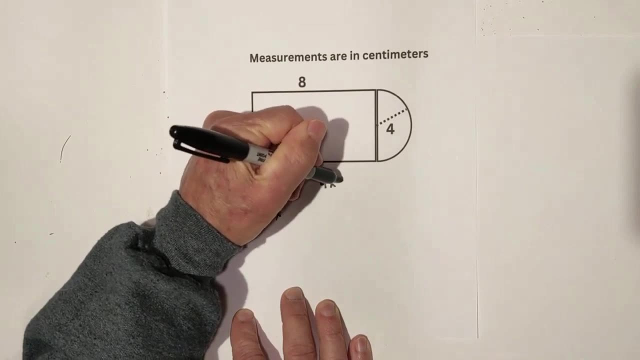 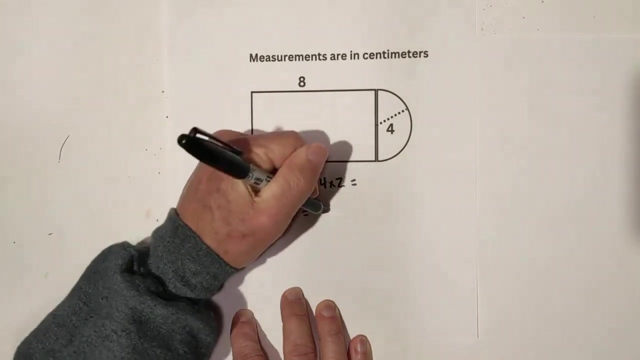 that the radius is going to be half of this line right here, because it's the diameter of the semicircle. so all we have to do is go 4 times 2, because the diameter is 2 times the radius, and that equals 8. when we multiply 8 times 8, that gives us 64, and the measurements are in centimeters. 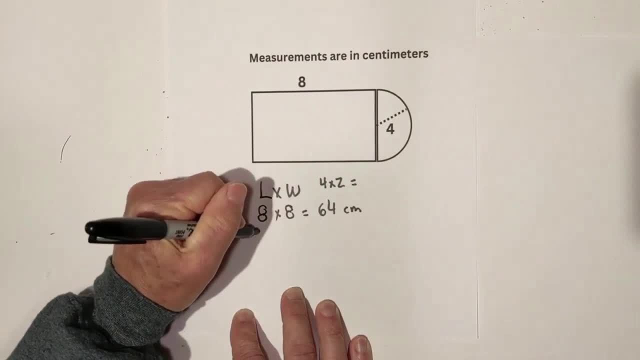 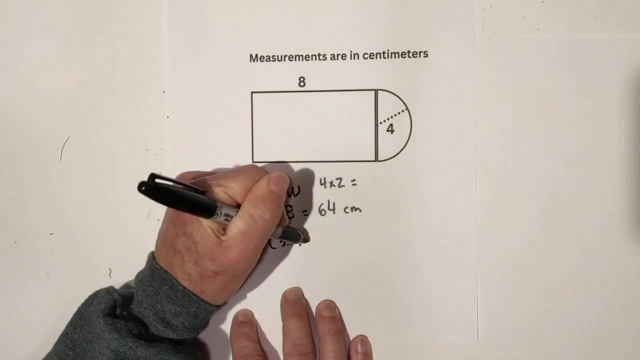 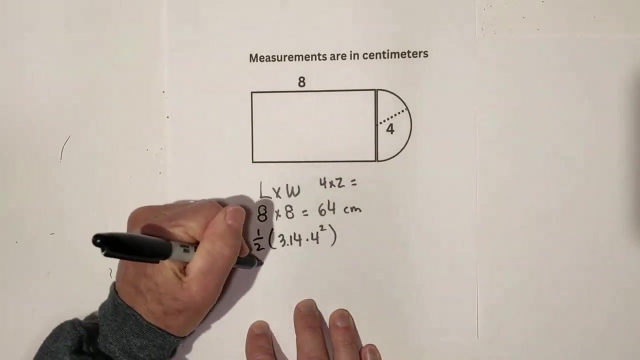 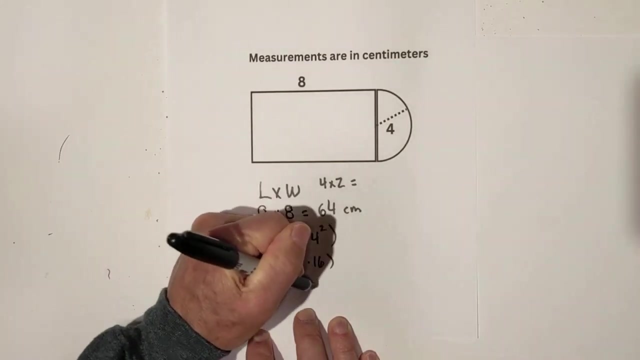 so now let's focus on this semicircle, and we can use one half times pi. i'm going to use 3.1, 4 times the radius squared, so we have 4 squared. let's work what's in the parentheses. first, one half times 3.14 times 16. okay, when you multiply 3.14 times 16, that gives me us 50.24. now i'm going. 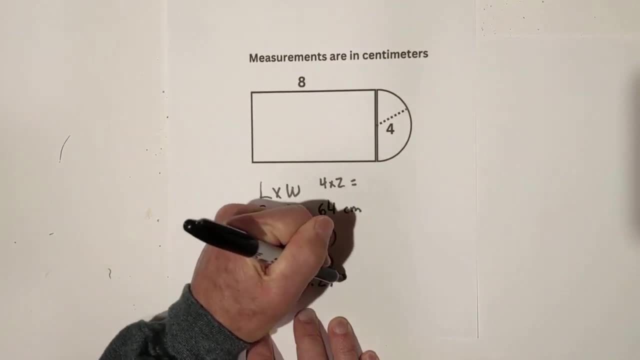 to multiply that by one half and that gives us 64, and the measurements are in centimeters, which you 25.12, so this will be in centimeters. so now all we need to do is add these two together. i'm going to bring down the area of the rectangle. that equals 64.00. okay, so far, so good. when we add: 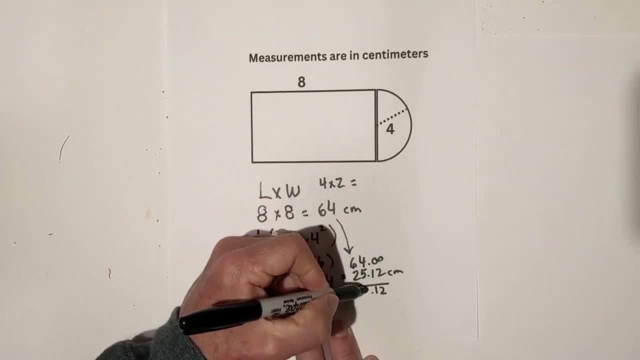 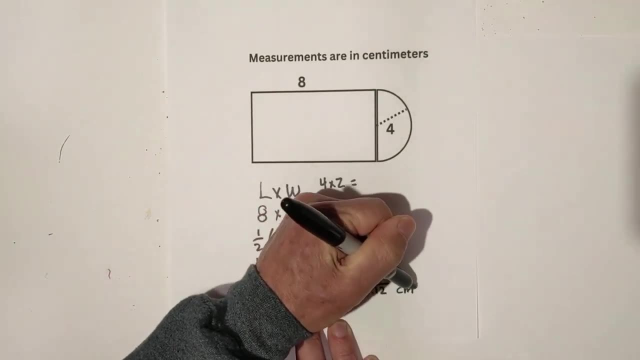 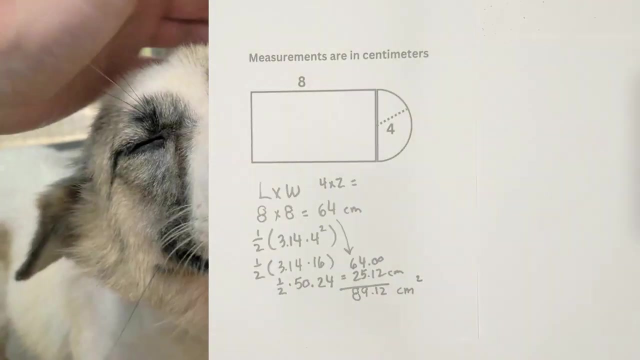 these: that's 2, that's a 1, 4 times that's 9 and then that's 8, 89.12. and remember it is centimeters and area is always square. i hope that was helpful. thanks for watching and remember. 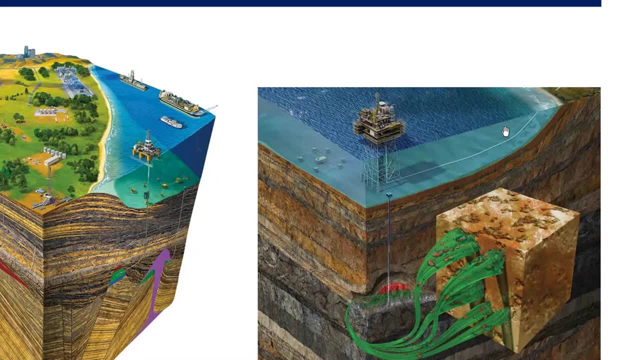 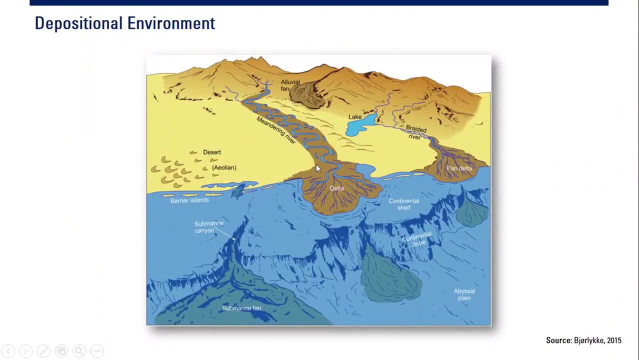 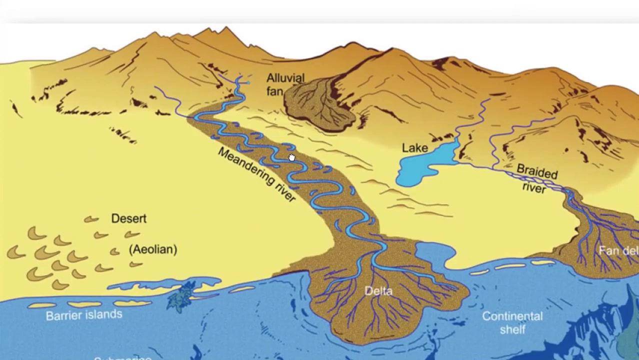 Okay, so that's the oil and gas reservoir, But many years ago, the reservoir is actually this environment. Okay, before it turns to be a reservoir, they are actually: some of them are river, Some of them are delta And some of them are lakes. 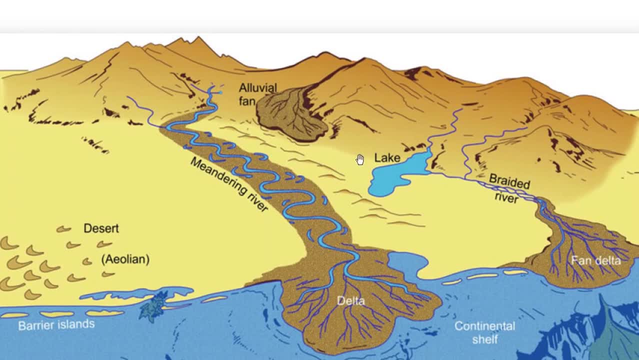 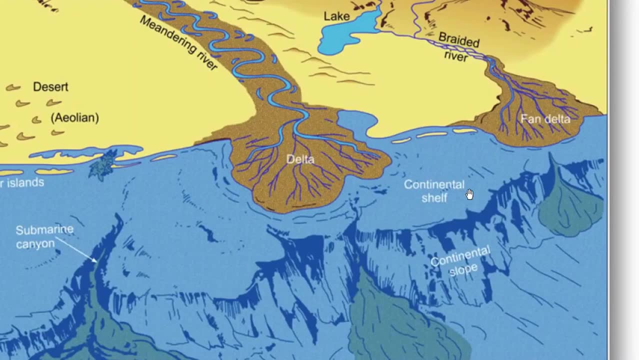 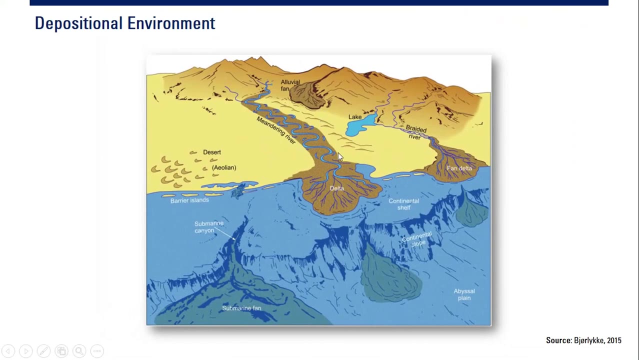 Because before they turned to be reservoirs they were Alufiel Fan, Braided River Fan, Delta, Continental Shelf and so on and so forth. Okay, so they will become reservoirs in the future. So yeah, some people say it's thousands years ago or million years ago. 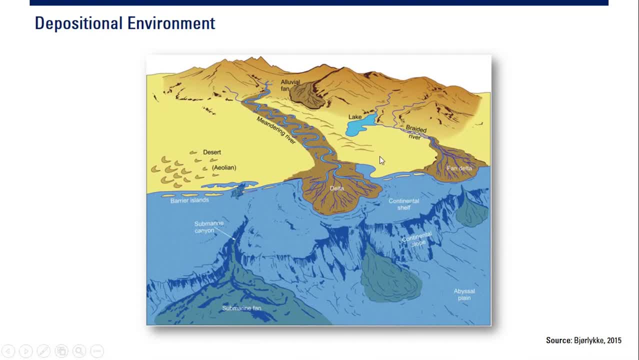 We are not sure, But before they turned to be reservoirs they were actually here: Submarine Fan, Continental Shelf, Delta and so on and so forth. And of course they will have different properties Because they come from different depositional environments. 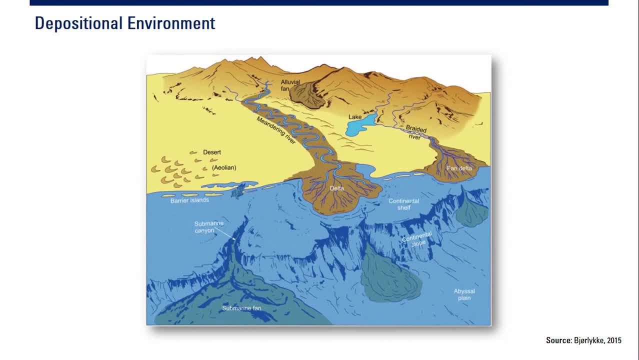 And, as reservoir engineer and reservoir simulator, we need to understand the depositional environment of our reservoir. And, as reservoir engineer and reservoir simulator, we need to understand the depositional environment of our reservoir. And, as reservoir engineer and reservoir simulator, we need to understand the depositional environment of our reservoir. 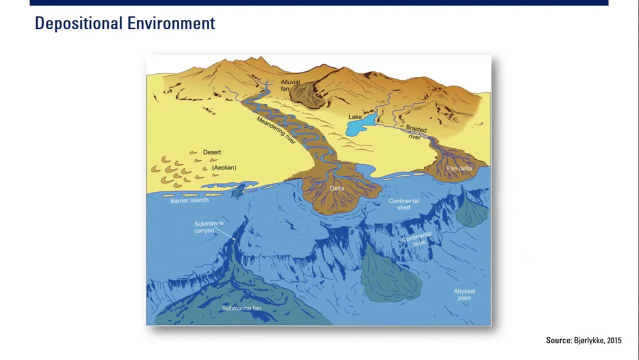 So if we want to simulate reservoir previously, which previously was river, it will have different properties with reservoir that actually was a lake. So if we want to simulate reservoir previously, which previously was river, it will have different properties with reservoir that actually was a lake. 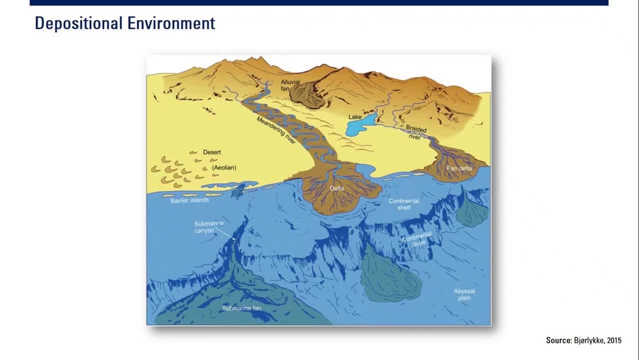